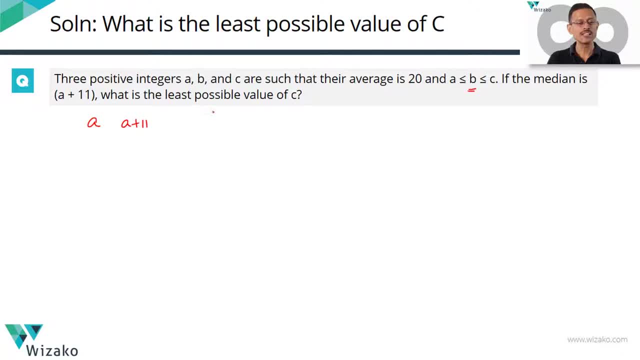 It cannot be lesser than b. So when you are trying to find out the least possible value for c, let's make c to be equal to b. This is the theoretically least value possible for c, So compute the value that, so a is equal. 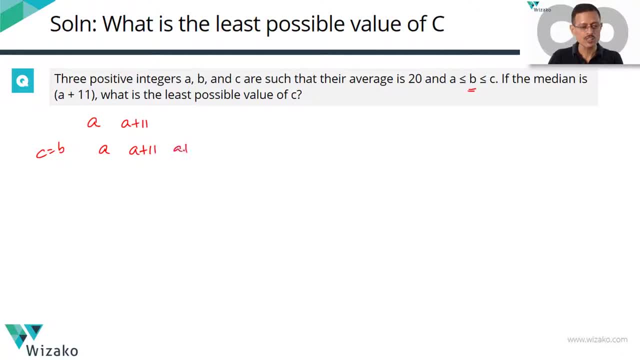 to a. b is equals to a plus 11, c is equal to b, which is also a plus 11.. The sum of these three values is equal to 60. So that makes it as 3 a plus 11.. plus 22 equals 60. Or 3a equals 60 minus 22,, which is a 38. Which boils down to the fact that 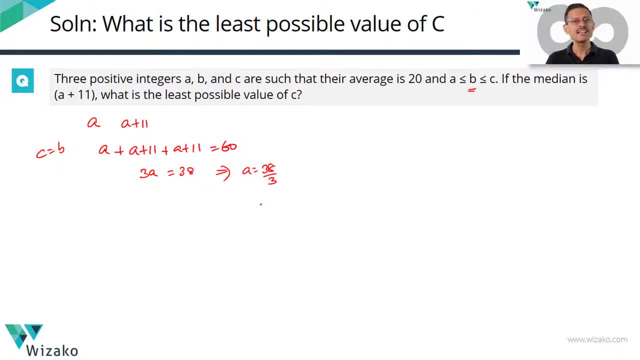 a is equal to 38 by 3.. a is 38 by 3, which is not an integer, which means b and c, which are 11 more than that, are also not going to be integers. So this is the condition that fails when we take c. 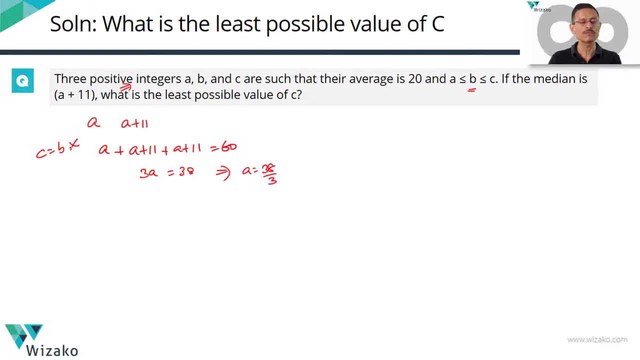 to be equal to b. That's not going to work, So this is ruled out. We're trying to minimize c. When c was equal to b, we got the theoretical minimum, which is 38 by 3 plus 11.. It's actually. 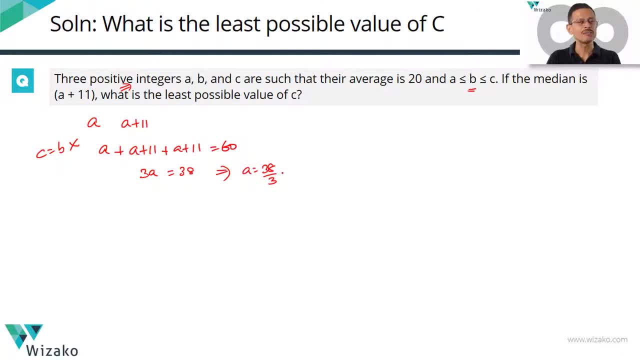 a 12.33 plus 11.. That's the least possible value for c, But because it's not an integer, we could not go with it. We're still trying to minimize c, So what we'll do is we'll give c as little more. 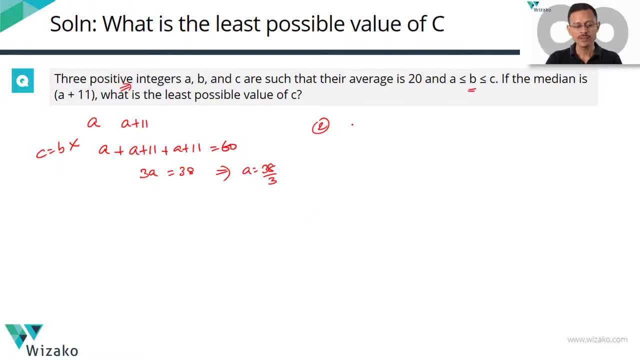 than b, as we can. So in iteration 2, what we're going to do is we're going to make c to be equal to b plus 1 and check out whether we're able to get values which are integers. a is a number. 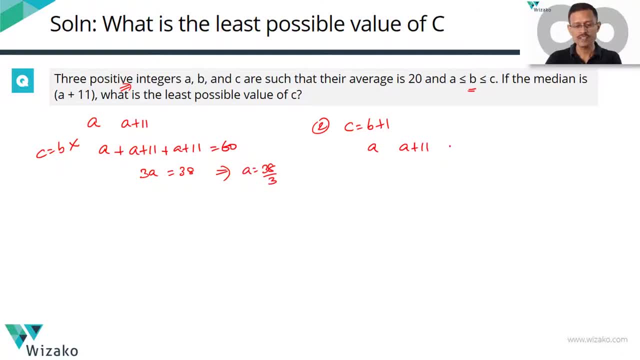 a plus 11 is the value of b. c is equal to b, b plus 1,, which is a plus 11 plus 1,, which is a plus 12.. Some of these three values should be equal to 60. So what we have here is 3a plus a 23.. Take it to the right-hand side: Makes 3a to 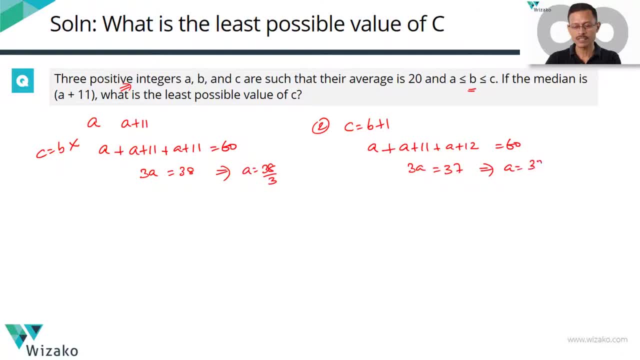 be equal to 37. Implies: a is equal to 37 by 3.. Same thing: a is not an integer, So c will not be an integer. This is also ruled out. Let's look at the third possibility We're trying to minimize. 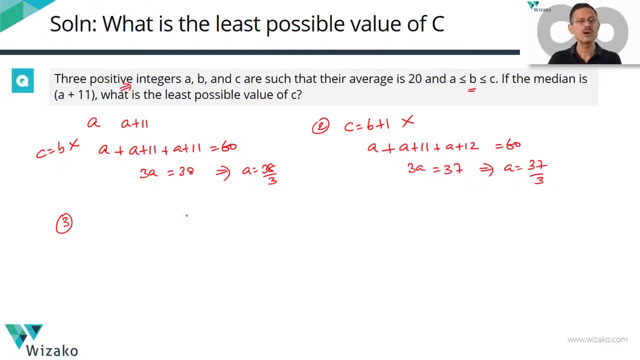 c, When c was equal to b plus 1, it did not work. Let's give 1 more than that. Let's make c to be equal to b plus 1.. Let's give 1 more than that. Let's make c to be equal to b plus 1.. Let's give: 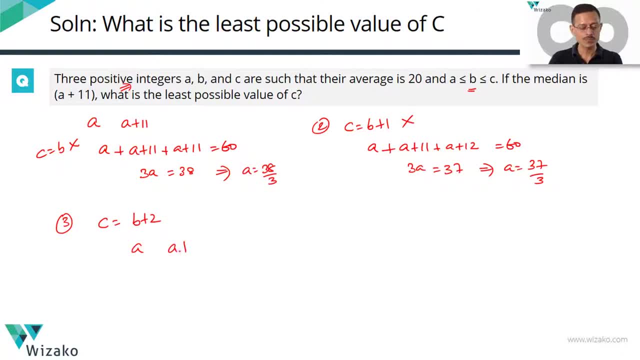 a plus 2.. Let's check out what happens. a is known. a plus 11 is the second number, which is the value of b. c should be 2 more than b, which is a plus 13.. So sum of all of these values is: